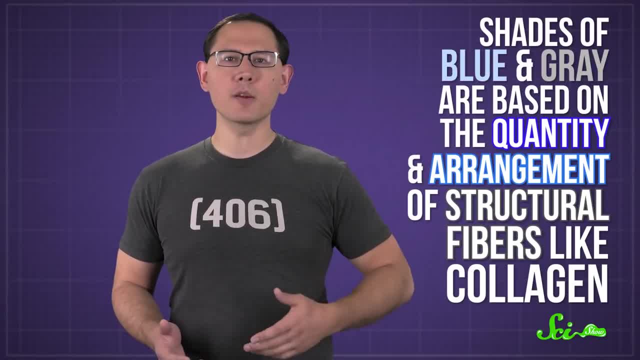 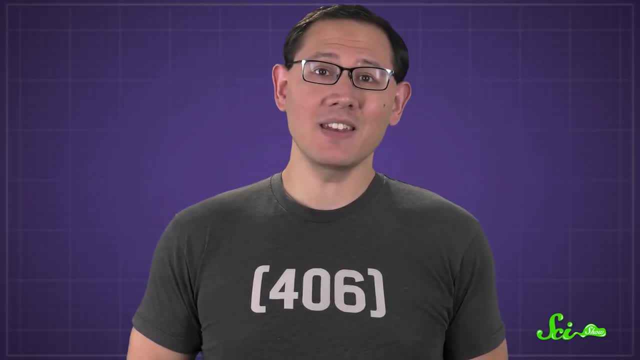 But melanin isn't the only thing that causes melanin, The whole story. Shades of blue and gray are based on the quantity and arrangement of structural fibers like collagen, which scatter light in slightly different ways. But even then, what you ultimately end up with is different amounts of light entering different colored eyes. 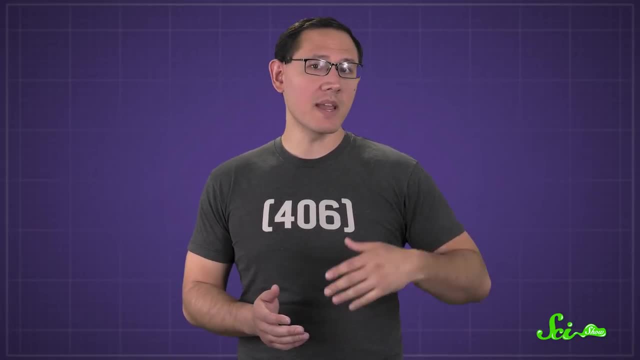 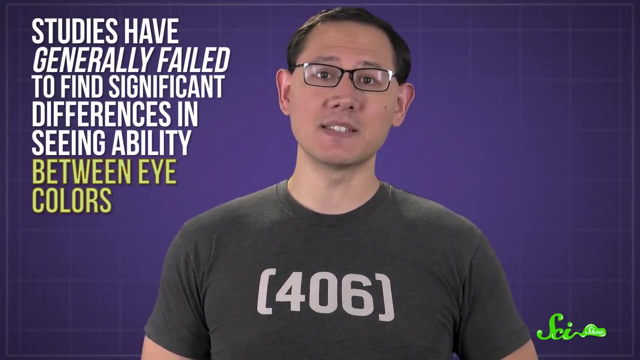 So you might think those eye colors see things differently, like one might have better vision, But the long and short of it is… not really. Studies have generally failed to find significant differences in seeing ability between eye colors, Although people with lighter-colored eyes may experience more discomfort on a sunny day. 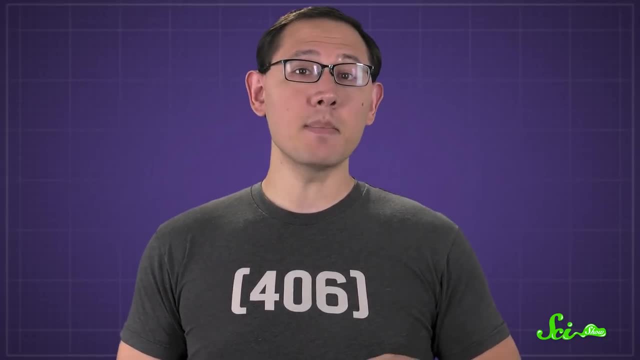 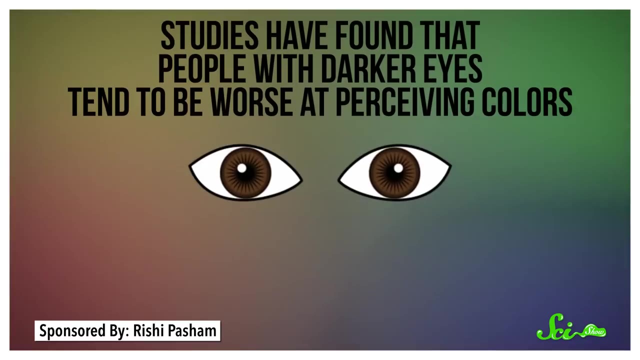 thanks to that whole more-light-in thing. Some biologists think that may mean they can see better in dimmer conditions, like when it's cloudy or at night, But so far this hasn't been conclusively demonstrated. Interestingly, studies have found that people with darker eyes tend to be worse at perceiving colors. 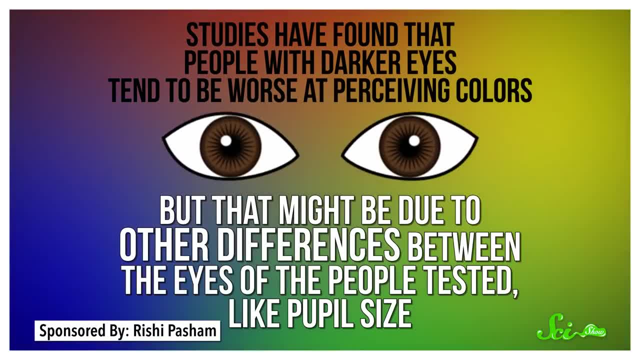 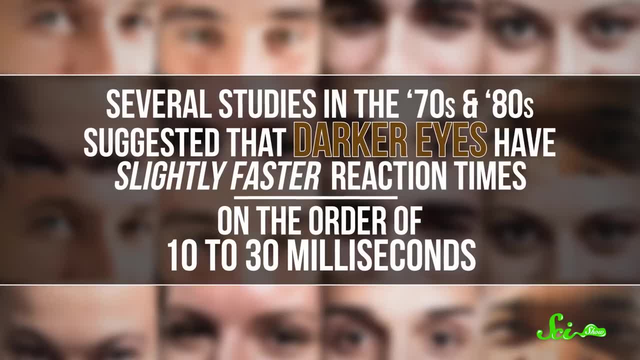 But that might be due to other differences between the eyes of the people tested, like pupil size. And one weird thing that keeps popping up is a difference in athletic performance between different eye colors. Several studies in the 70s and 80s suggested that darker eyes have slightly faster reaction times. 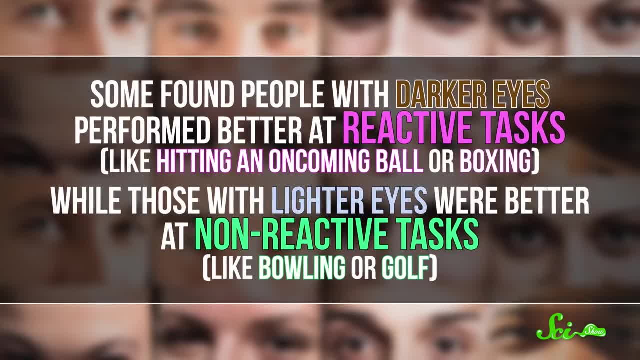 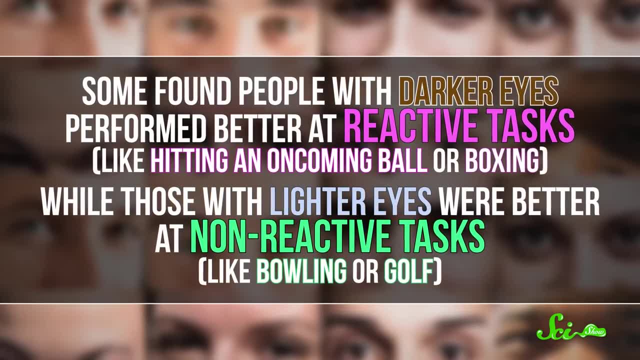 on the order of 10 to 30 milliseconds. Some found people with darker eyes performed better at reactive tasks like hitting an oncoming ball or boxing, while those with lighter eyes were better at non-reactive tasks like bowling or golf, And that might have something to do with the amount or quality of light that melanin absorbs. 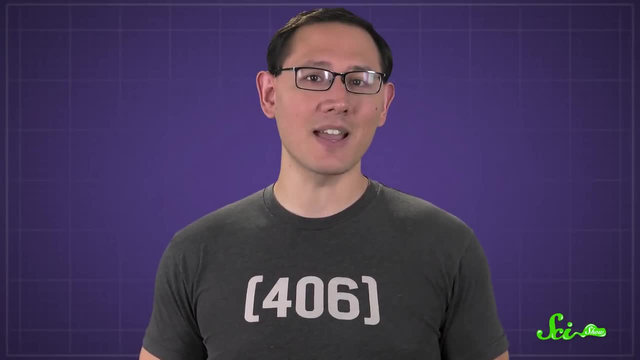 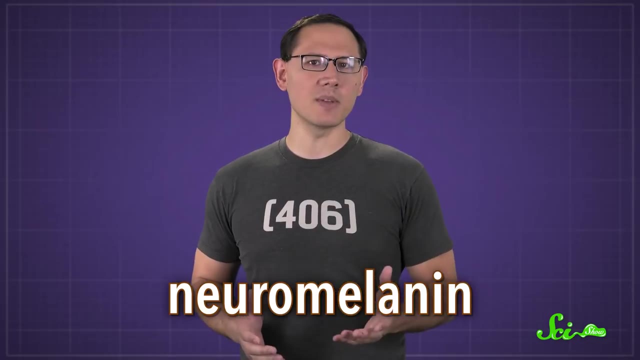 But the most likely hypothesis for this actually has little to do with eyesight. It's thought that melanin in the iris correlates to levels of neuromelanin in the central nervous system, a related set of pigments that may help speed up neuronal signaling. 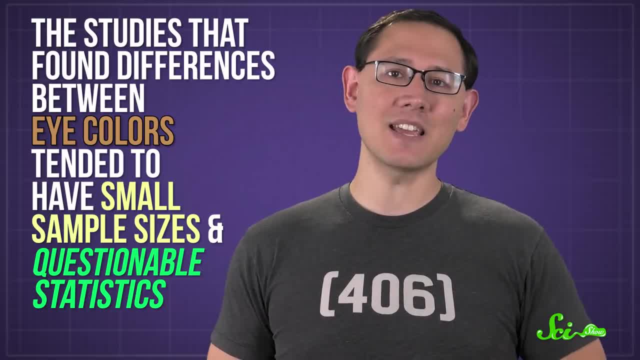 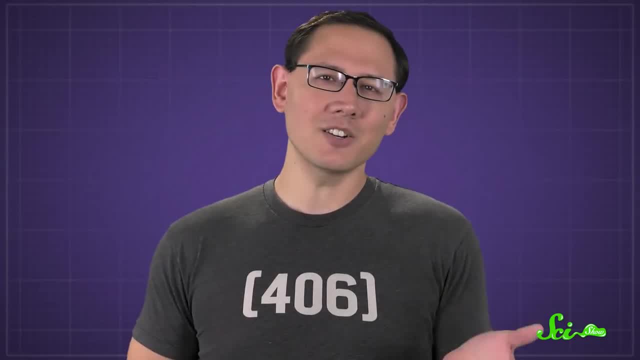 And, in general, the studies that found differences between eye colors tended to have small sample sizes and questionable statistics. More recent replication attempts haven't gotten the same results, So it's hard to say if iris color really affects vision. And even if it does, most experts think the effects are really slight. 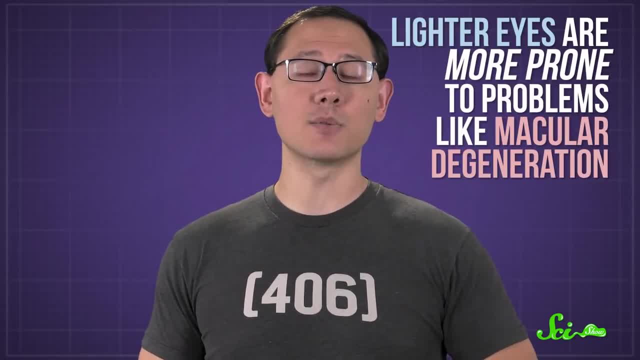 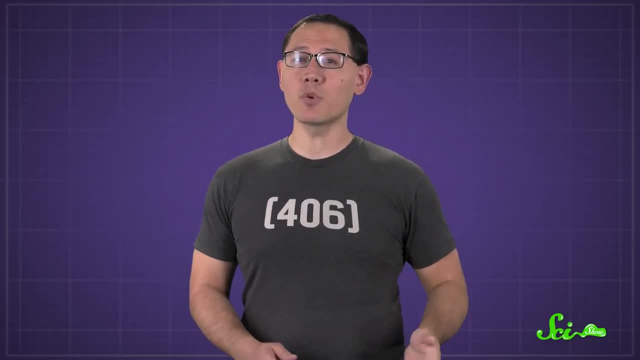 What iris color does impact is eye health, as lighter eyes are more prone to problems like macular degeneration- the failing of the region of the eye that lets us see objects directly in front of us, And that means people with blue eyes might want to be a bit more careful about wearing.